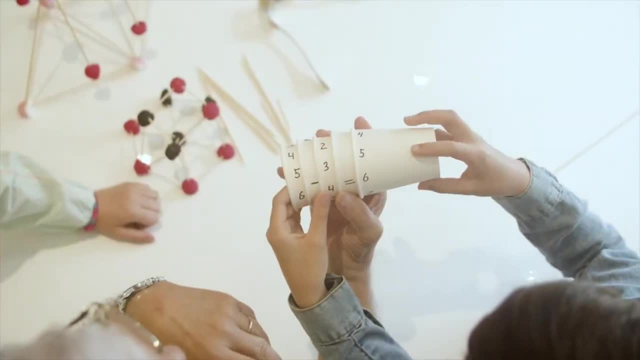 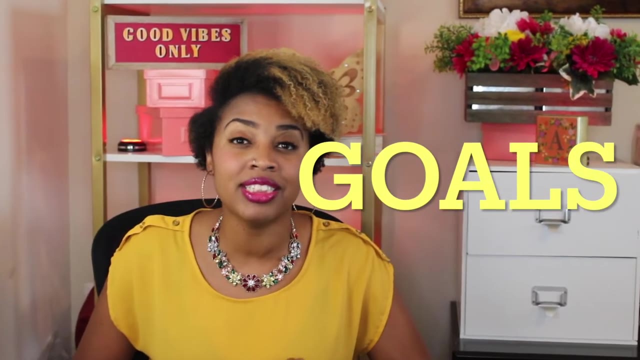 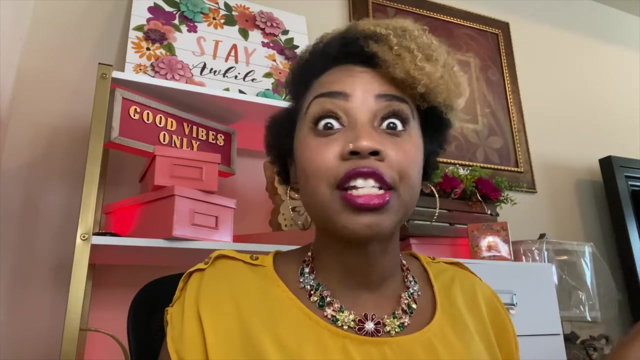 Math fluency is developed through automaticity. Kids must be able to recall basic math facts both quickly and accurately. It is proven that children that are fluent in basic math flags do better on standardized tests, in addition to having less anxiety and less stress with doing higher computation. You certainly can't do fractions if you don't know how to multiply. 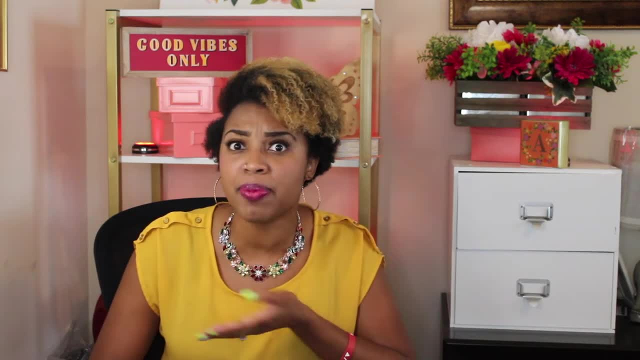 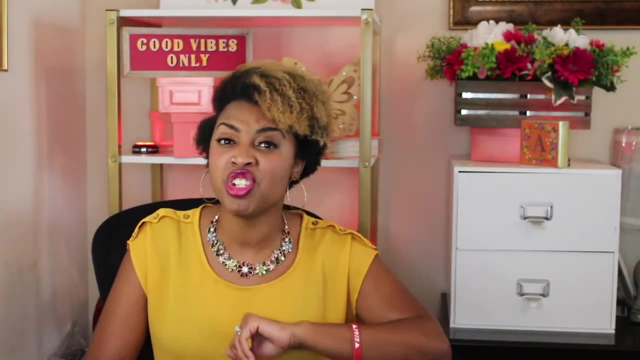 I see this all the time. Kids can't even do fractions because they're simply spending all their time sitting there doing skip counting or even drawing array models. Today, I want to share with you one game that will help children become fluent with all four operations. 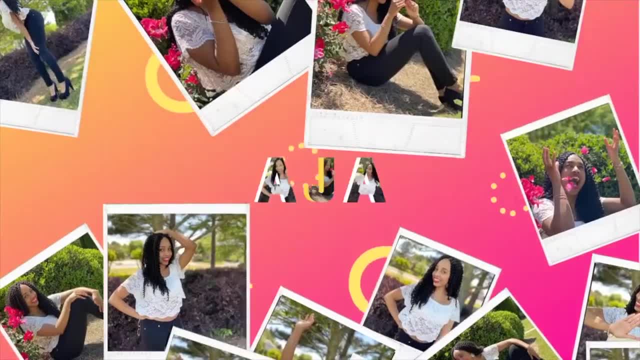 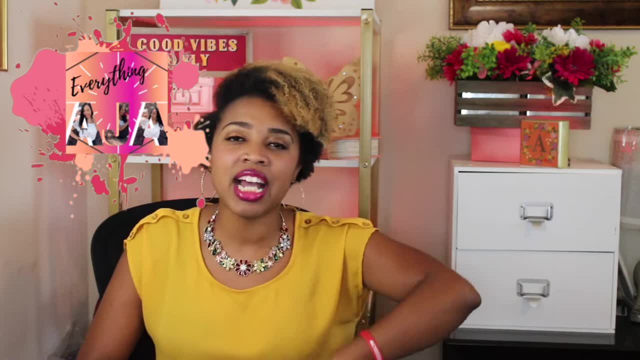 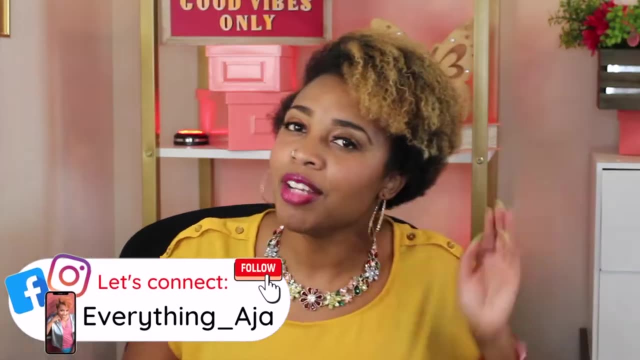 Hey fun people, Welcome back to Everything Agile If you're new here, hi, I'm Aja Here on Everything Agile. I help parents and teachers, just like you, make learning as fun, strategic and easy as possible. If this sounds like you, then what are you waiting on? Go ahead. 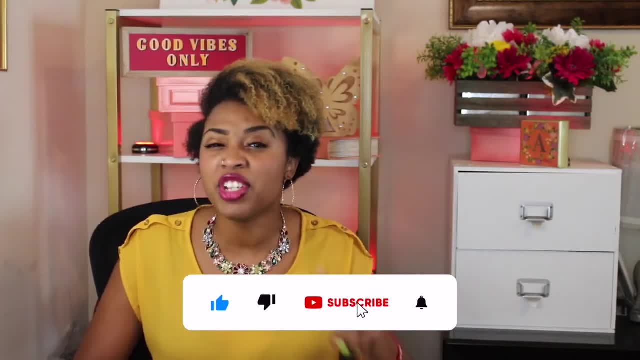 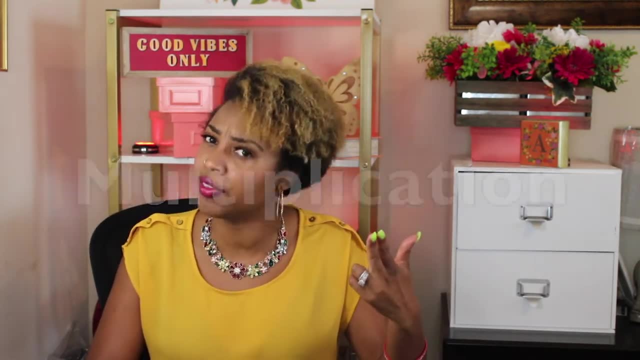 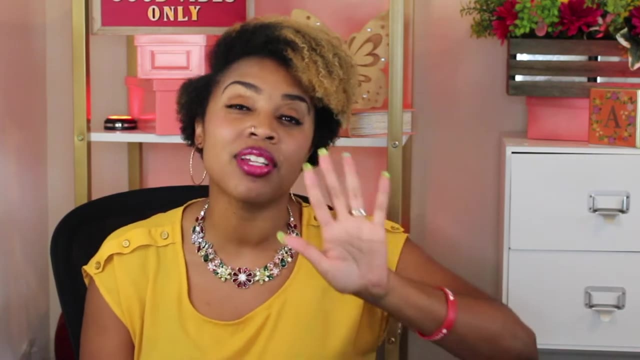 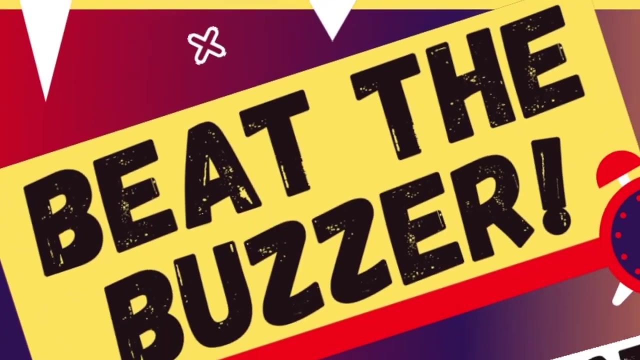 and subscribe. Today I want to share with you one game that can be beneficial for any child learning math. The game I want to share with you is called Beat the Buzzer. Beat the Buzzer is a digital game that can be played in the classroom and even online. That means you can play with. 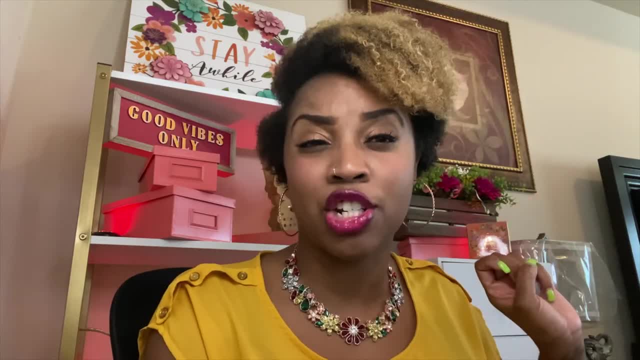 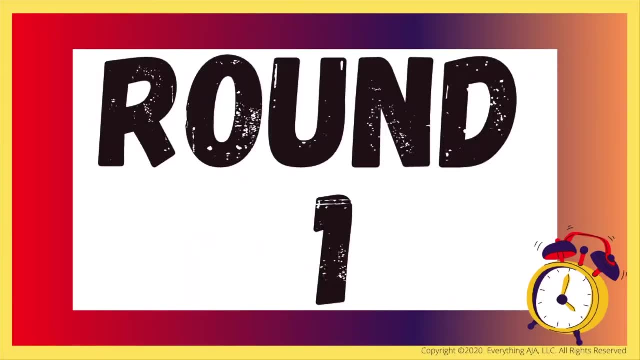 your entire class in the classroom, during small group instruction, in centers and even online during distance learning. Zoom games for the win. So the amazing thing about Beat the Buzzer is that it can be played solo-dolo. This is perfect for parents. Beat the Buzzer. 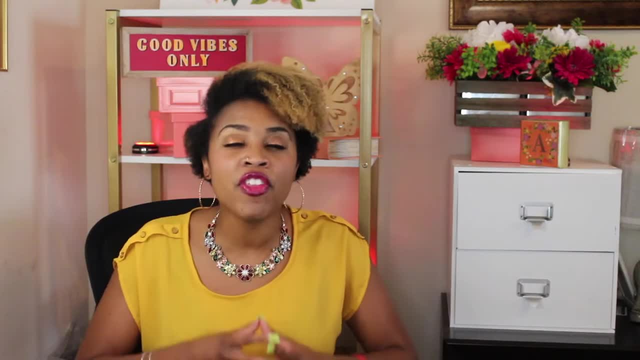 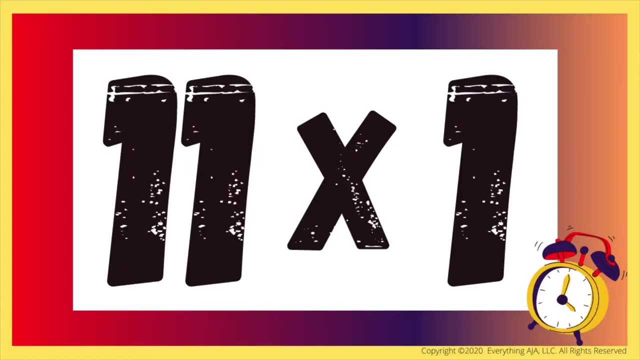 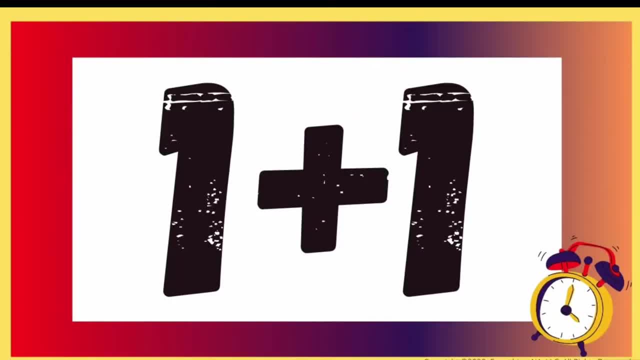 miss more than one round, then they're out. If they miss more than one round, then they're out. If they miss more than one round, then they're out. They've gotten two answers per round. You can always make this more challenging and make it one. If a child gets out, they. 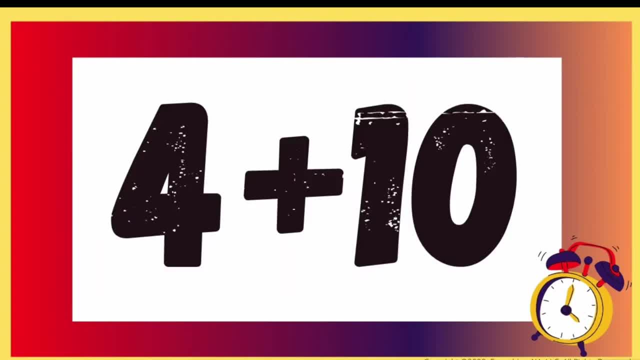 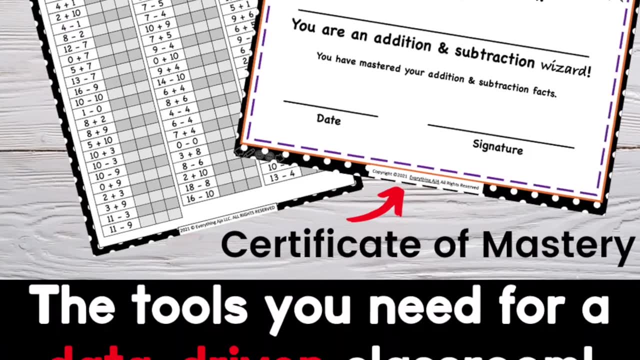 did not beat the buzzer and then they have to play again to beat their high score. This is how people can play it by themselves. The game also comes with a checklist with all the problems during each round. This way, kids can actually quiz themselves and mark.